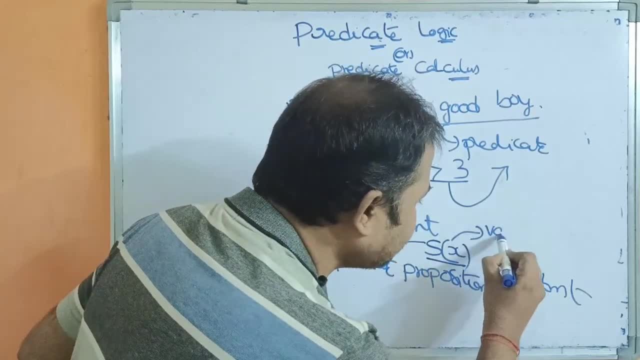 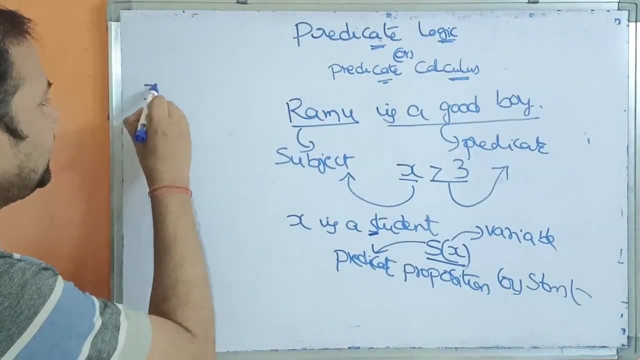 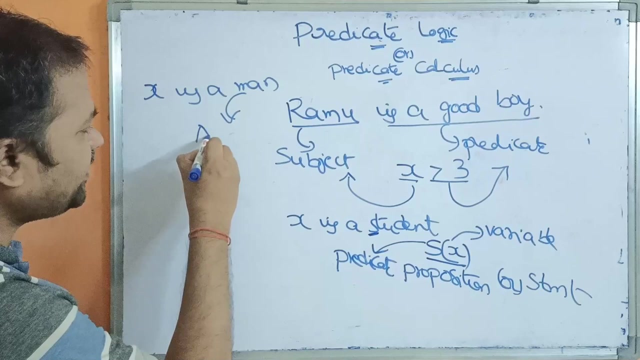 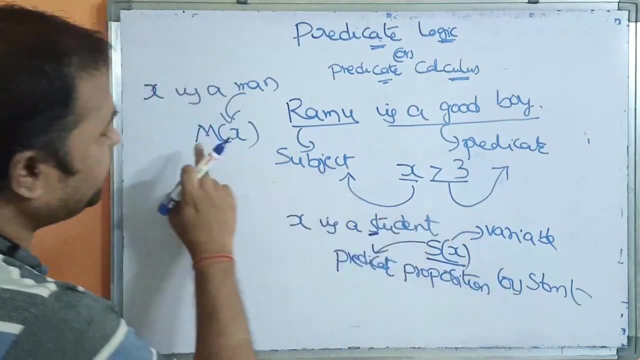 predicate, whereas this x is called as a variable. x is called as a variable. so let us take one more example. let me have a statement called x is a man, so this is represented with the help of here. man is starting with m, m of x. so m of x is called as preposition function or statement function. this m is called as predicate. 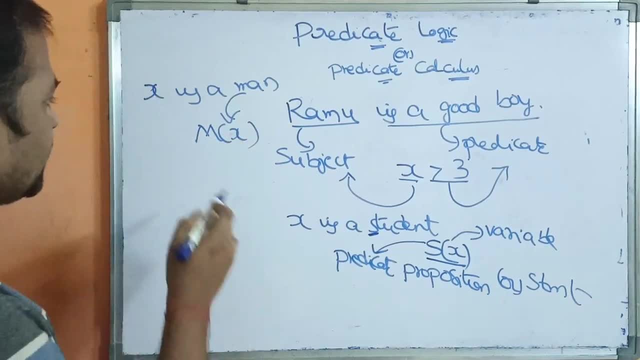 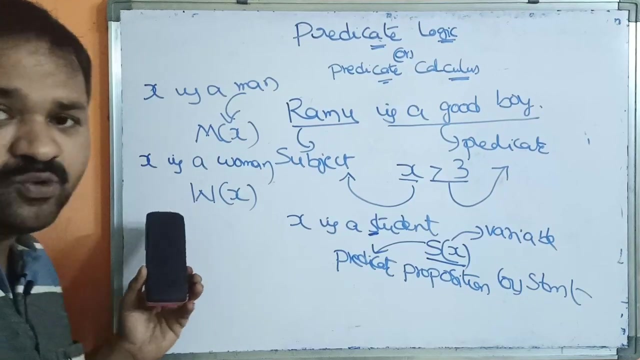 whereas x is called as a variable. okay, let us take one more example. so let me have a statement like this: x is a woman, so woman is starting with w. so here the statement function are preposition function is w of x. this w is called as predicate, whereas x is called as a variable. 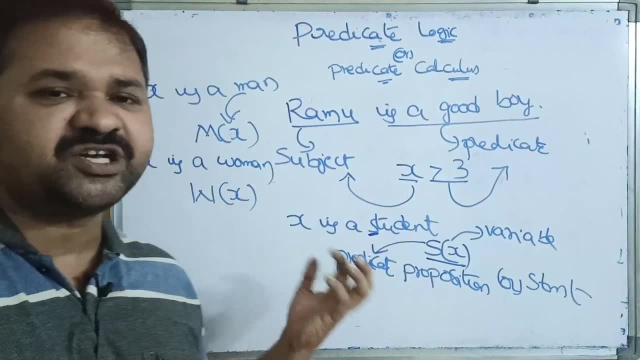 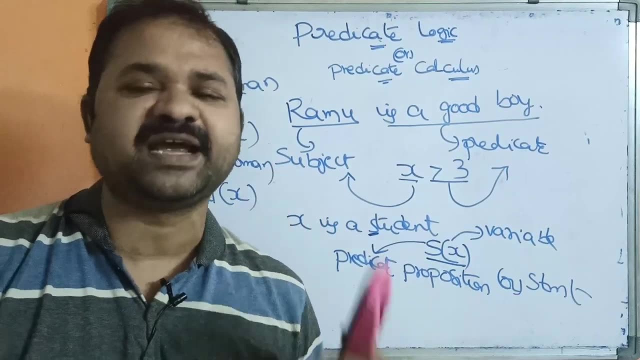 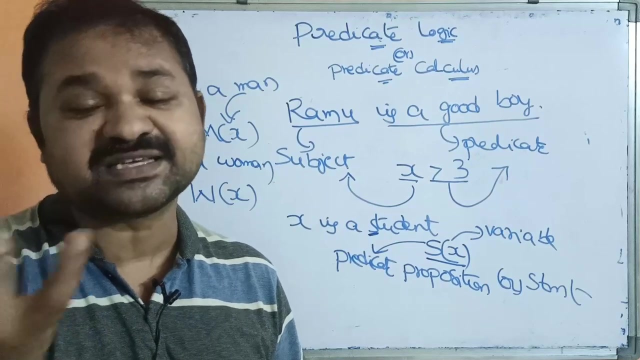 so this is about what is a statement function and what is a variable. here we can perform various operations. we can construct compound statement functions. we know what is a compound preposition. compound preposition means if the if we use as correctives, then it is called as a compound. 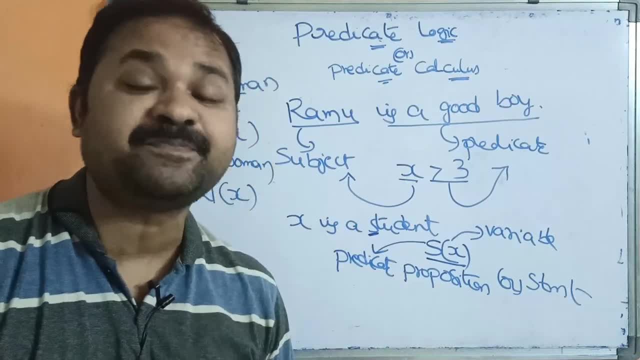 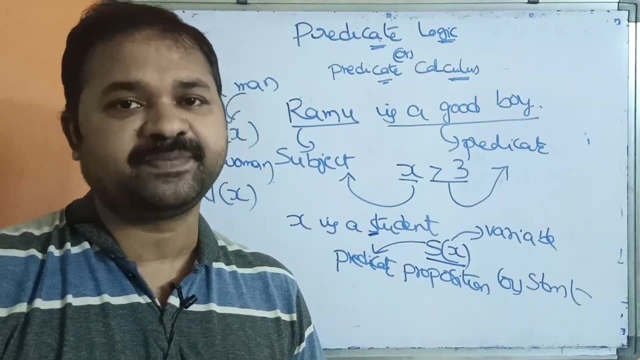 preposition. likewise we can have compound statement function, vì if we use as correctives in the statement function viz that is called as compartment statement function, we have different types of corrective, such as kind connect you or connect you, negation, connect you, implication, connect you by conditional. connect you likewise. 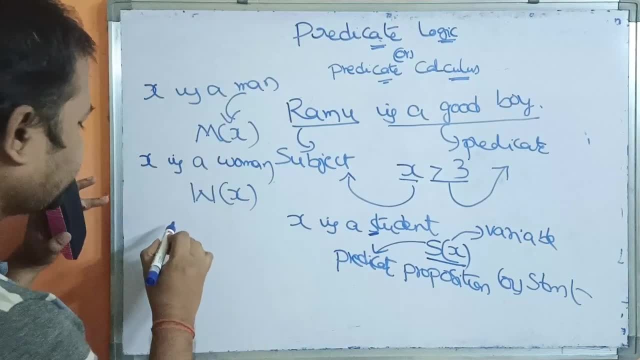 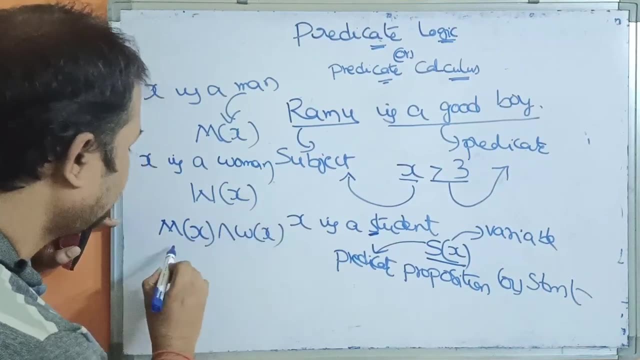 so we can have various compound statement functions such as m of x and w of x, yeah of x or w of x. so next one m of x, viz two wom of x and two one m of x. and, as you can see, when we use cond identities under connectives, 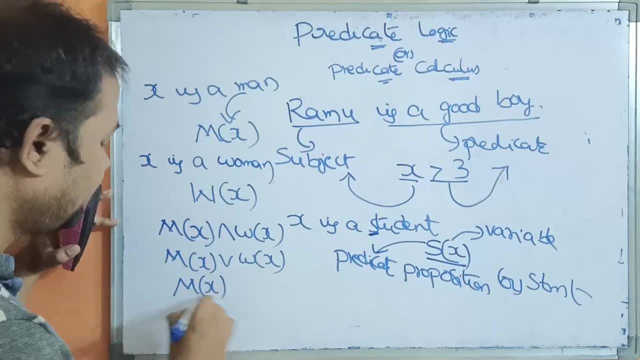 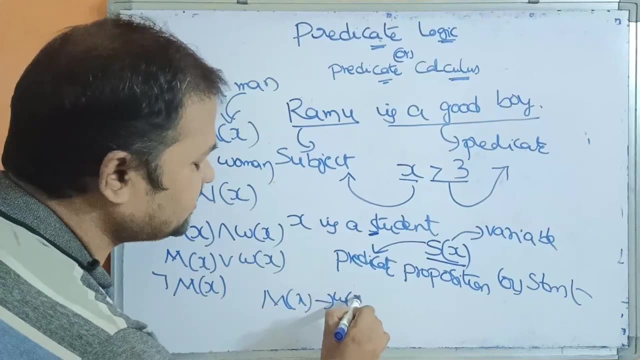 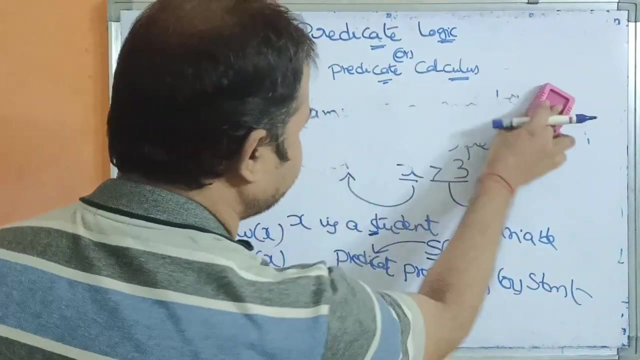 then when we complete- and we complete, we meet the next assignment: negation of m of x. next we can have m of x, implication w of x. likewise we can construct the various compound statement functions. now let us see about quantifiers mainly. we have two types. 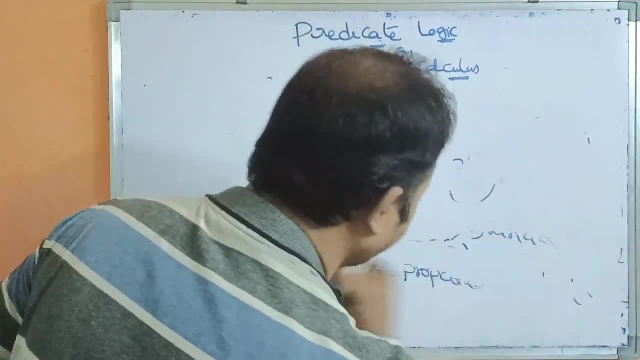 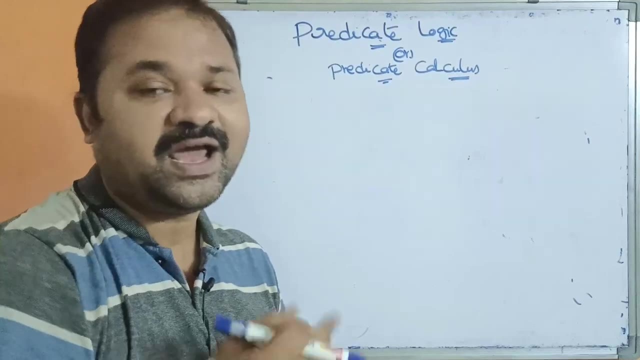 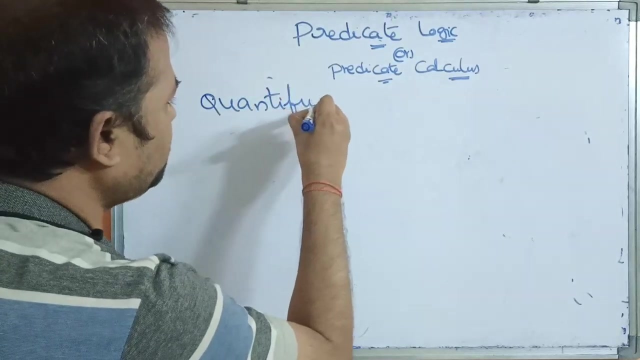 of quantifiers. are there quantifiers? okay, so till now we have seen about what is predicate, lossic and what is statement function, what is a variable and what is a compound statement function. now let us see about quantifier. quantifier, so we have two types of quantifiers. are there? 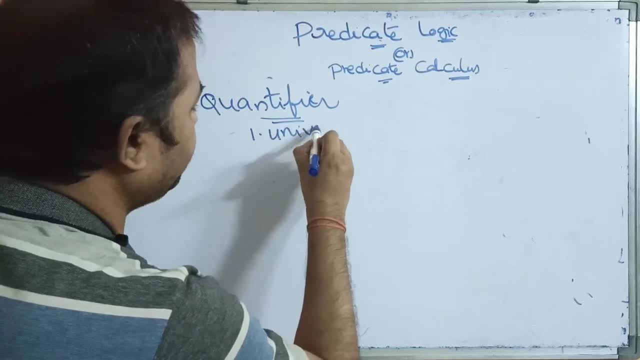 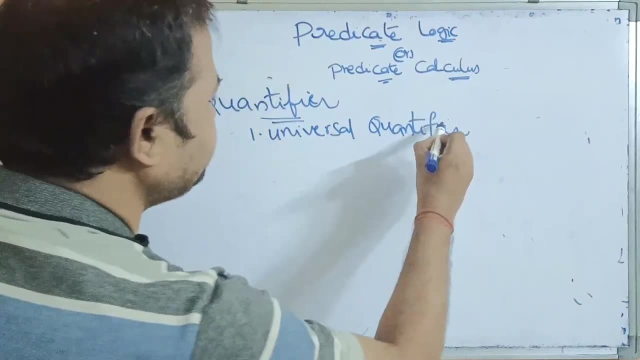 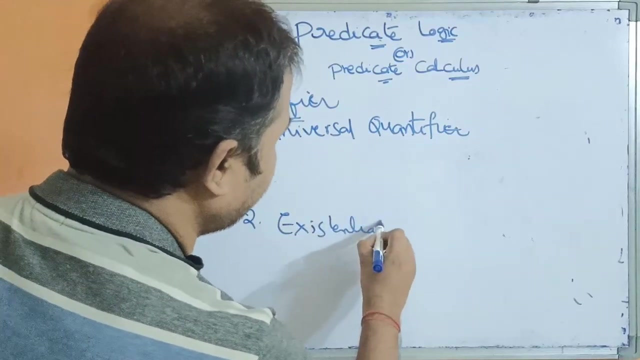 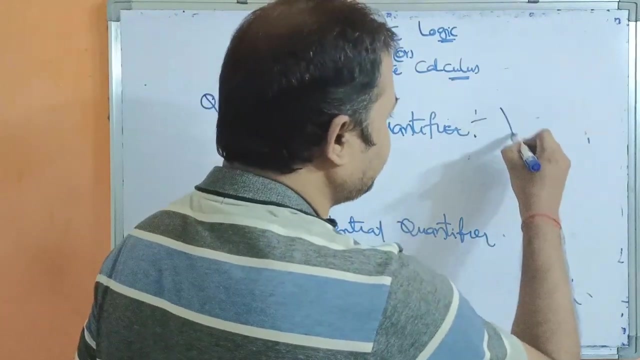 the first one is universal quantifier. first one is universal quantifier. second one is existential quantifier. second one is existential quantifier. second one is existential quantifier. let us see about universal quantifier. let us see about universal quantifier. universal quantifier is represented by the symbol reverse of a, so this symbol is pronounced as: 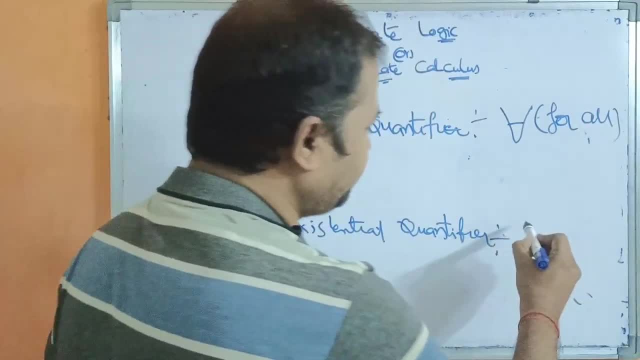 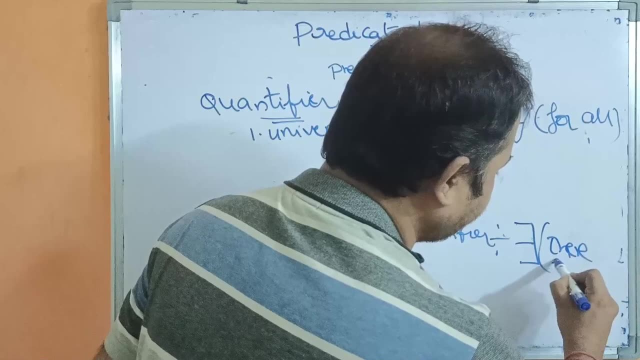 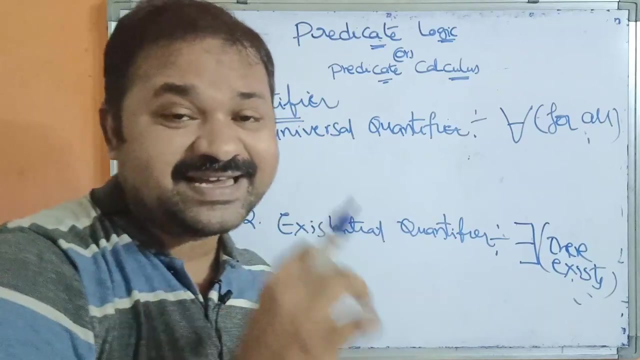 for all. various existential quantifier is represented by this reverse. reverse of a. the symbol is pronounced as there exists. the symbol is pronounced as there exists. now, let us see when we can use universal quantifier. if the sentence contains the praises such as for all. if the 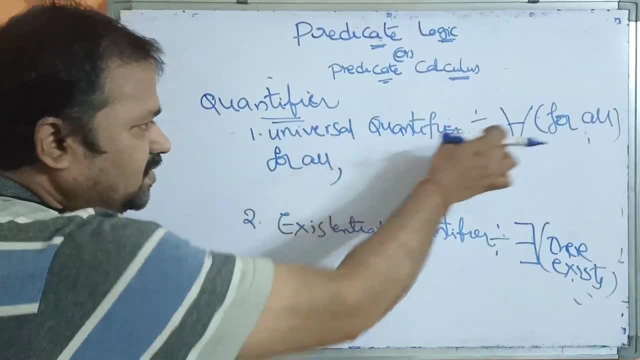 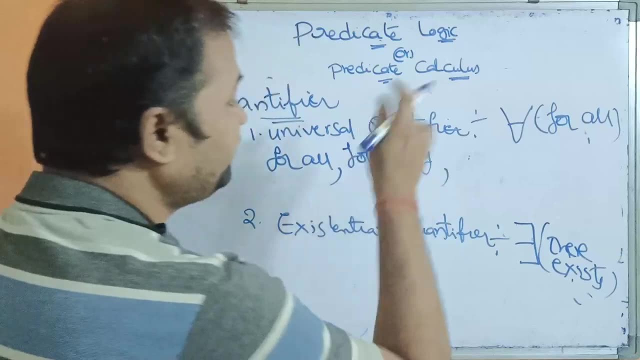 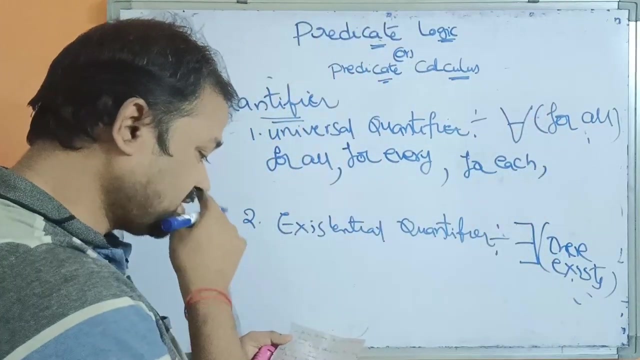 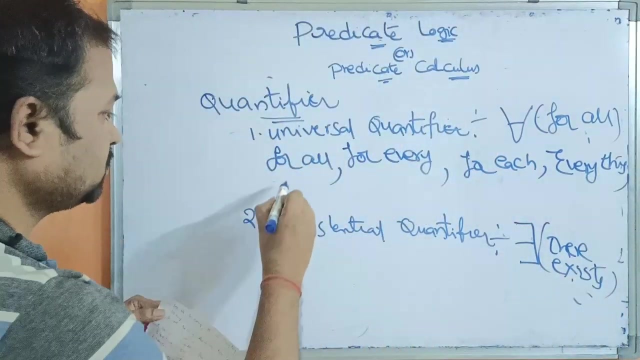 sentence contains for all, then we have to use universal quantifier. so likewise, if the sentence contains for every, for every or every, we have to use universal quantifier. so likewise, if the sentence contains each or for each, we have to use universal quantifier. if the sentence contains everything or anything, or for any, 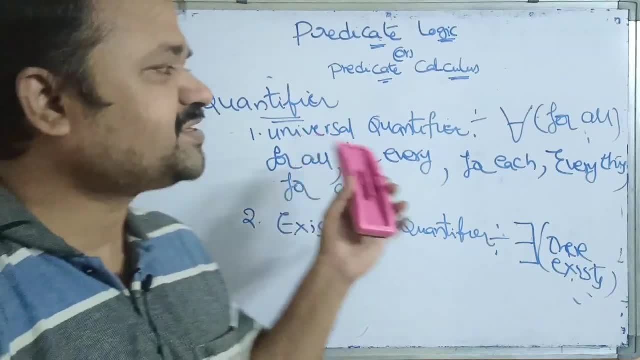 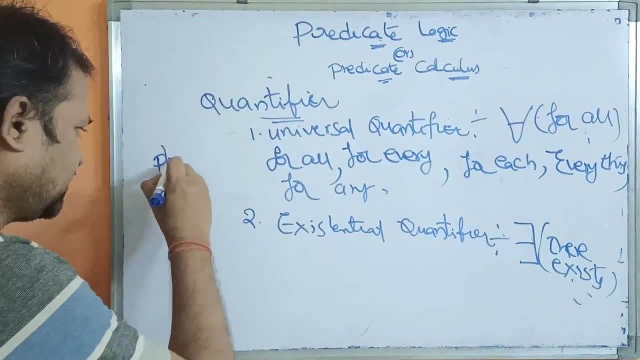 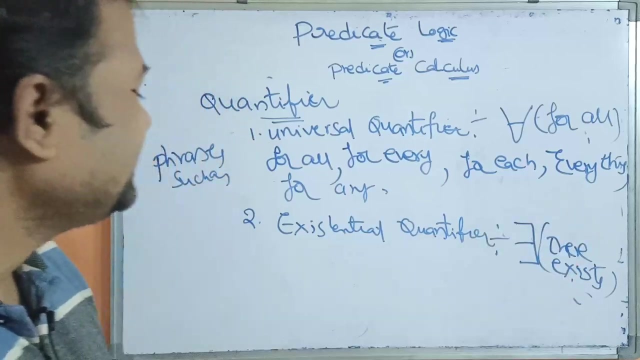 then we use this universal quantifier. so universal quantifier is represented by for all symbol, and if the sentence contains praises, words, if the sentence contains praises such as for all, for every, for each, anything, everything, for any, then we use the universal quantifier. now let us see about. 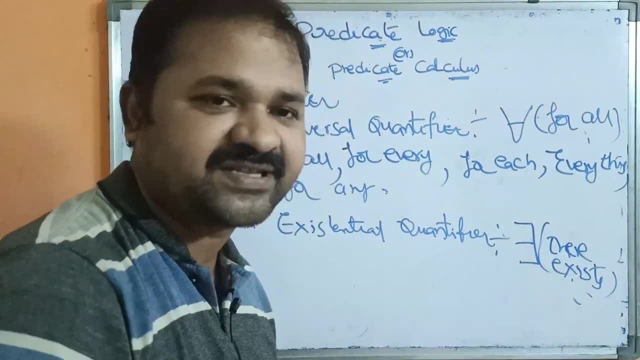 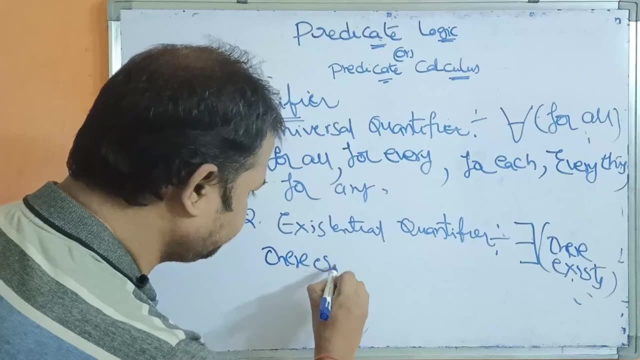 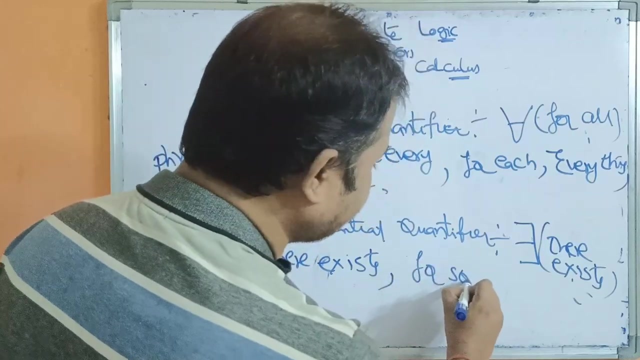 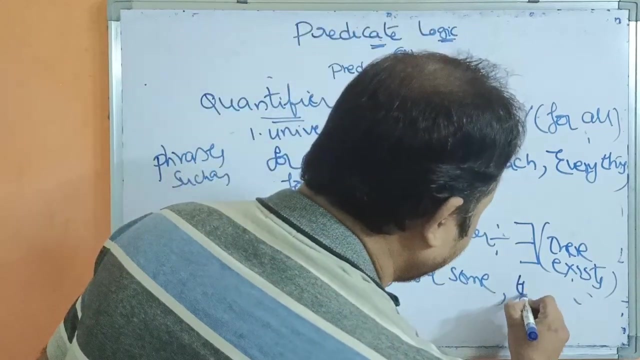 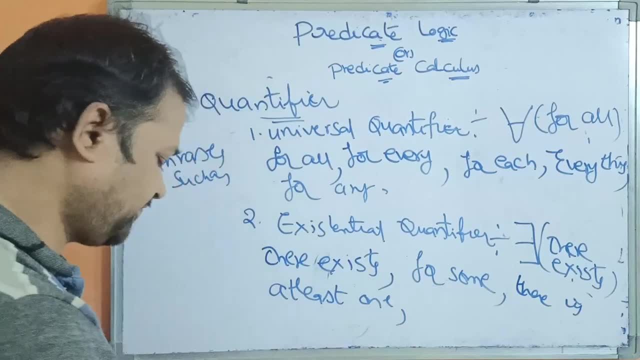 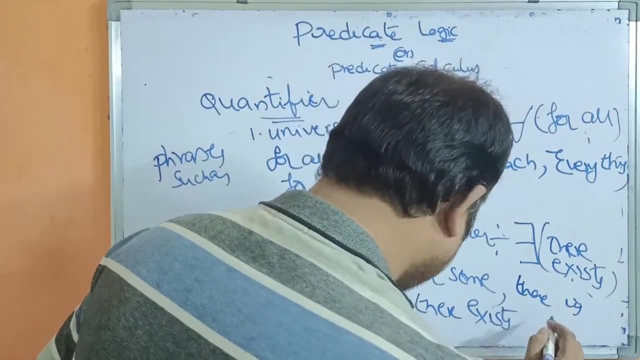 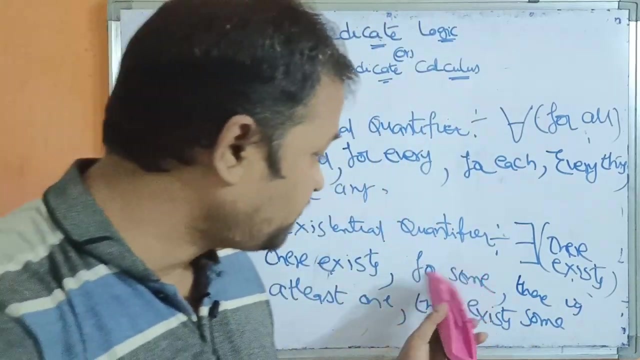 least one, then we have to use the existential quantifier. or if the sentence contains Lagis there exists, there exists some, there exists some. so if the sentence contains there exists or some, for some, there is at least one, there is at least one, or if the sentence contains there exists some, then we have 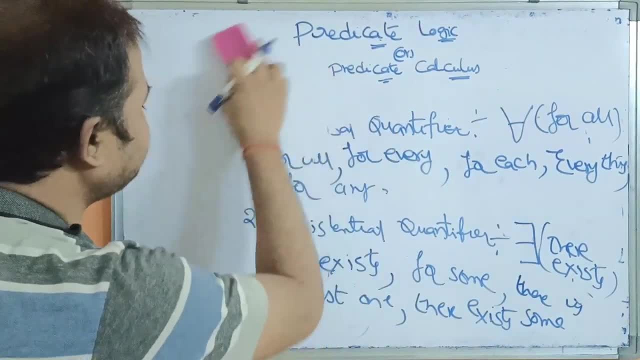 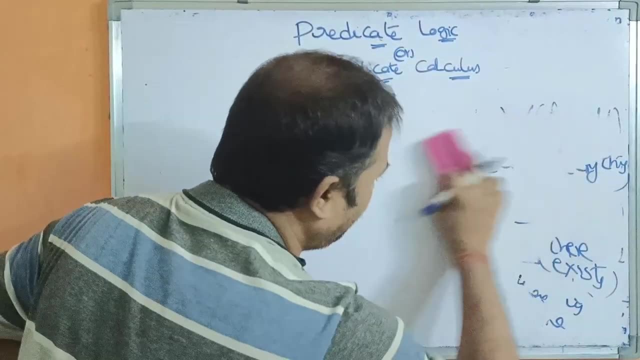 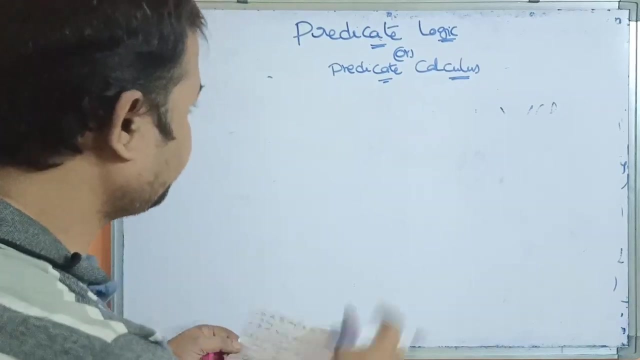 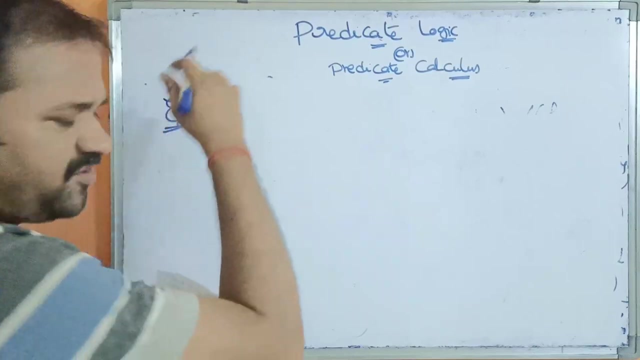 to use this existential quantifier. now we have three examples are there and it is represent these three examples with the help of the predicate logic, that means with the help of the 的 quantifies. so let us solve those three examples so that it predicate logic will be over example. but first let us see example one represent the following: 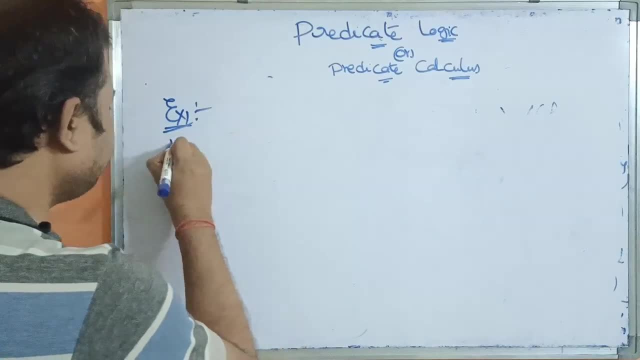 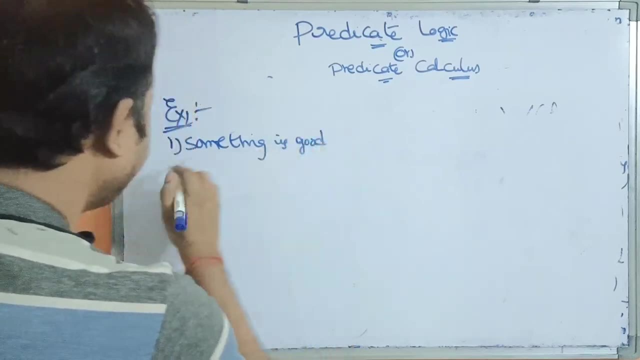 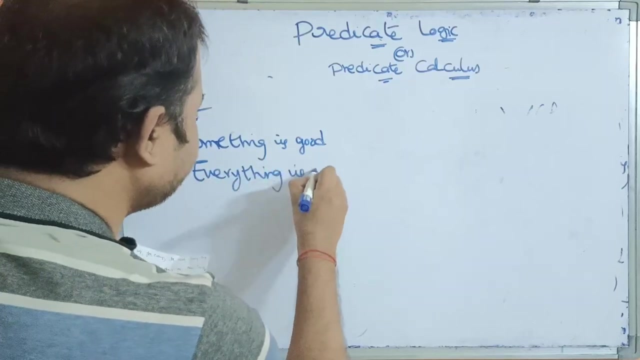 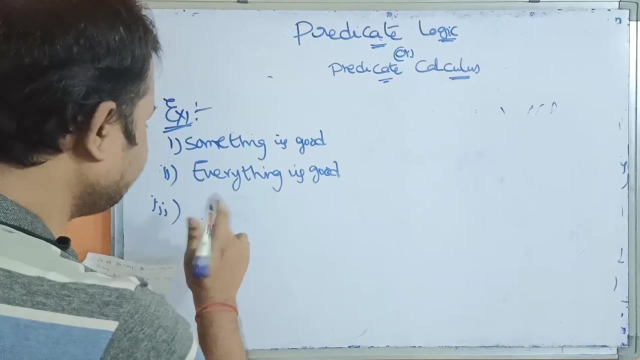 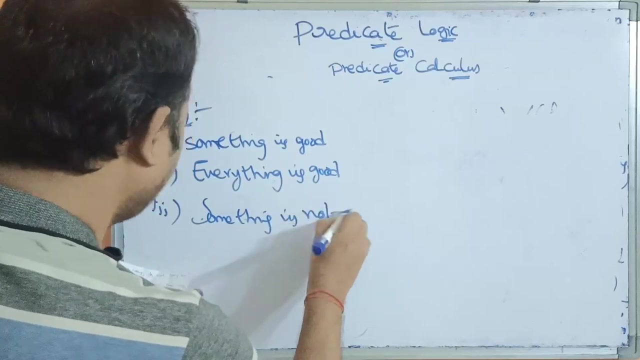 sentences in symbolic form. so first, two sentence: something is good, something is good. second sentence: everything is good. second sentence: everything is good. third sentence: something is not good. let us represent this statement. first: yeah, something is not good, something is not good. last one: nothing is good. last. 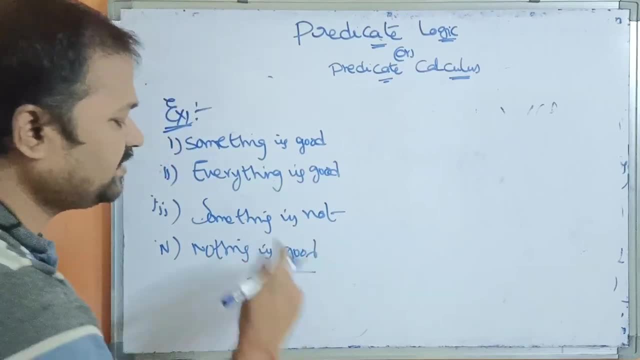 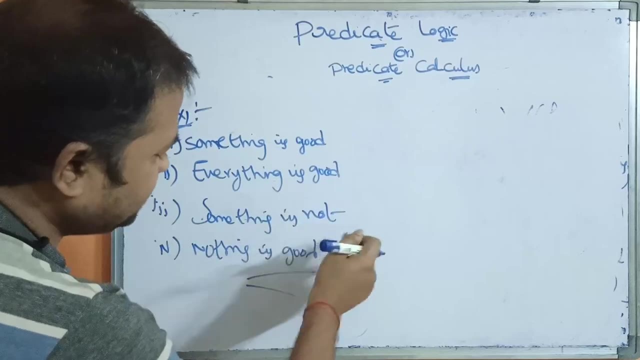 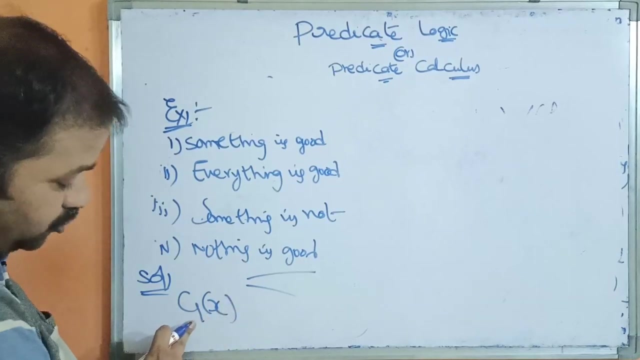 statement: nothing is good. okay, so we have to represent all these statements in the symbolic form using predicate calculus. okay, so here, in every statement we have, he is good, he is good, he is good. so let us represent that statement. okay. G of X, G of X. here G stands for good, X stands for x, X is good. 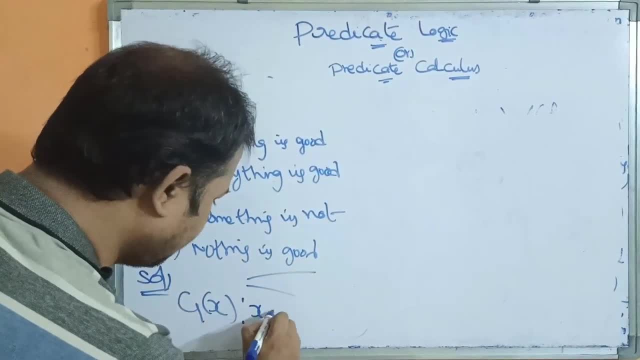 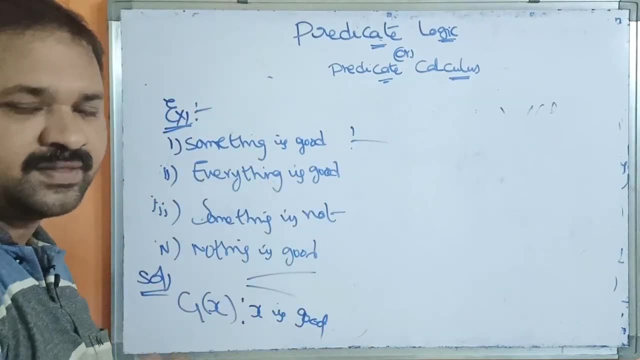 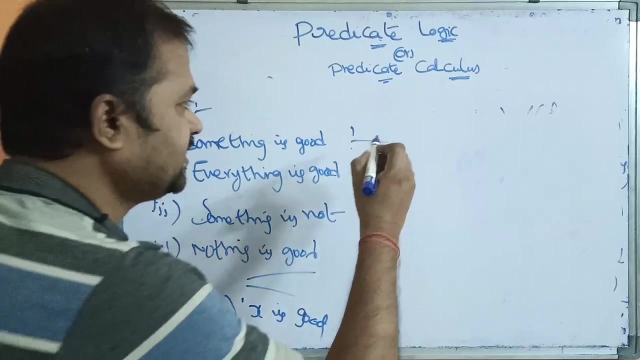 okay, this is nothing but statement function or preposition function. here we are representing with the help of what X is good. okay, let us represent the first statement. something is good. that means here the sentence contains sum. if the sentence contains sum, then we have to use as existential quantifier. So there exists x. Here we are using 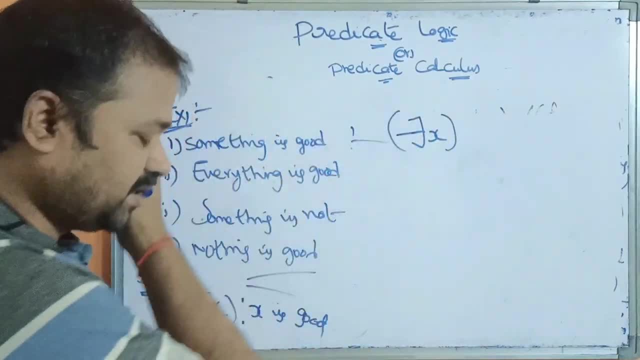 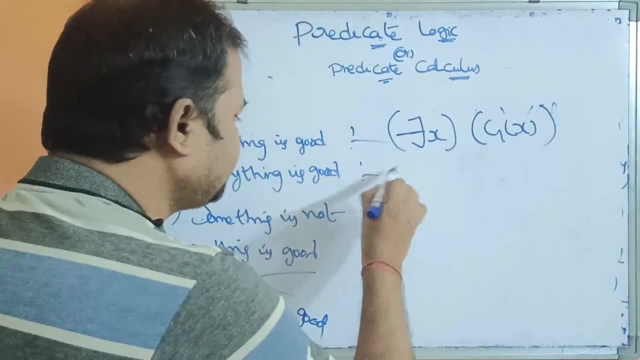 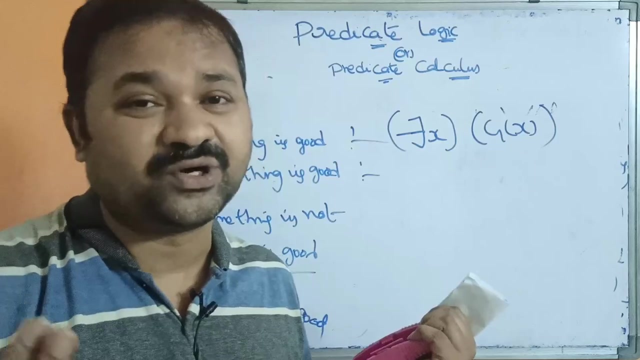 the variable x We have to place within the parenthesis. Good How to represent good g of x. Within the parenthesis write the function. Okay, Let us represent the second sentence. Everything is good. Everything means what? Anything, Anything, All, So all is good. So 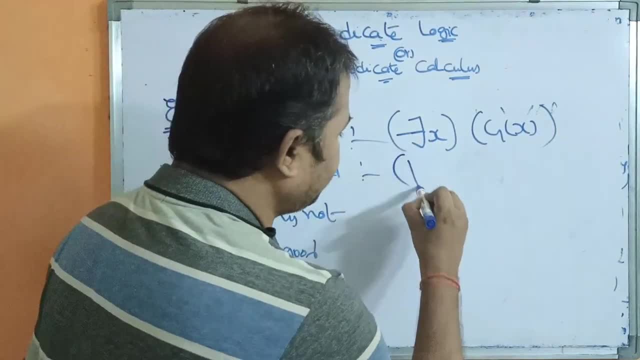 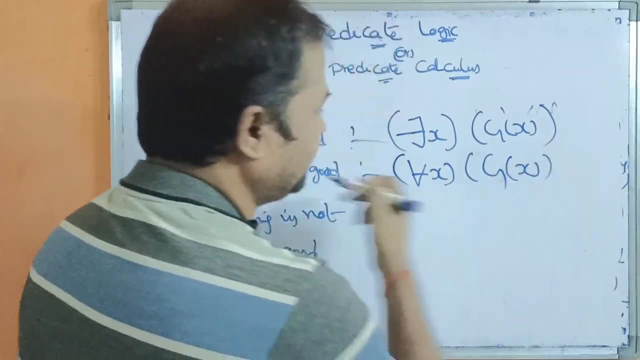 all means we have to use universal quantifier. That is for all x, For all x, all Everything is good, So g of x. So we can write like this: Okay, Next one. something is not good Here, something. 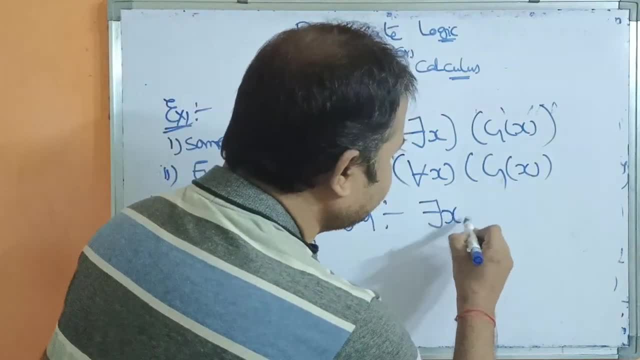 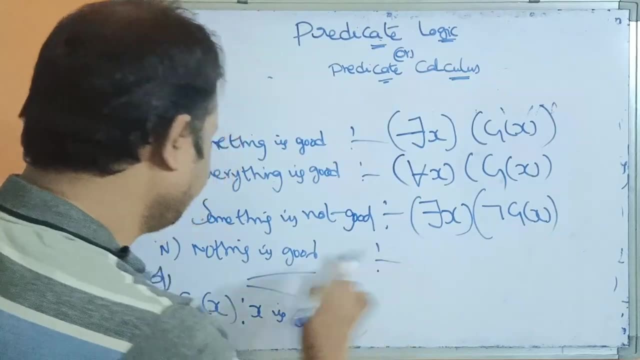 is not good, So something means we have to use this. There exists not good, So not good means we have to use this negation, quantifier, Negation. Okay, Nothing is good, So that means everything is not good. 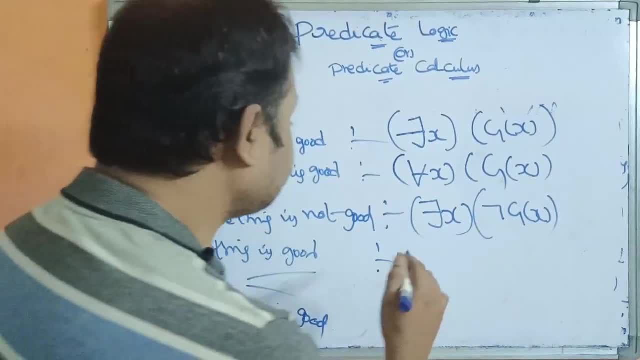 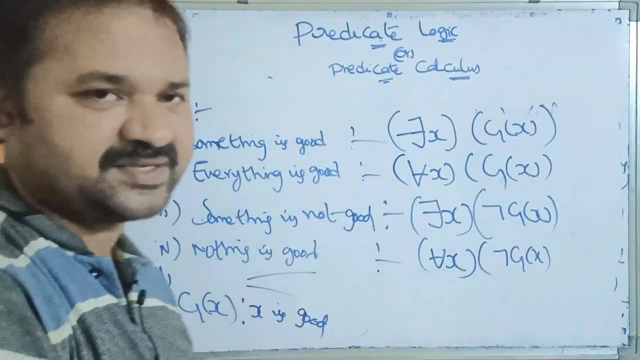 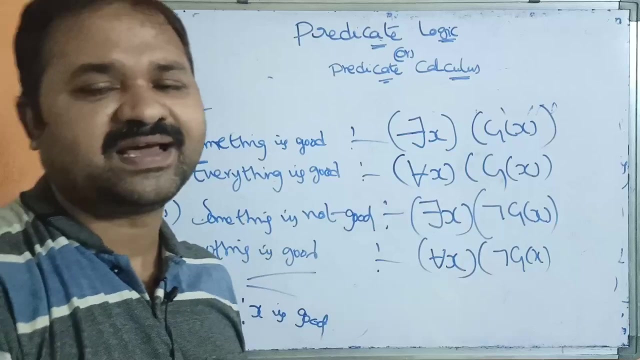 Everything is not good, All is not good, So all means for all x, Everything means for all x. So not good means not g of x. So in this way we can represent In the examination. some sentences will be given, So we have to construct, We have to represent them with the. 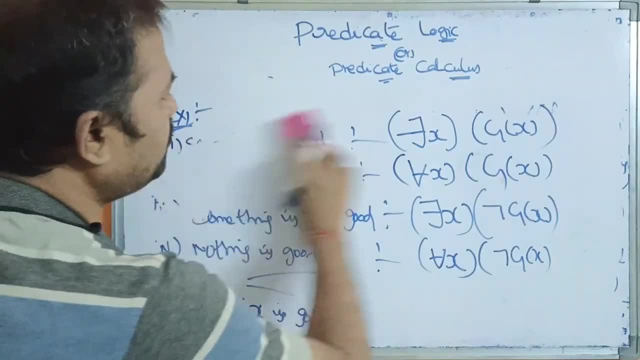 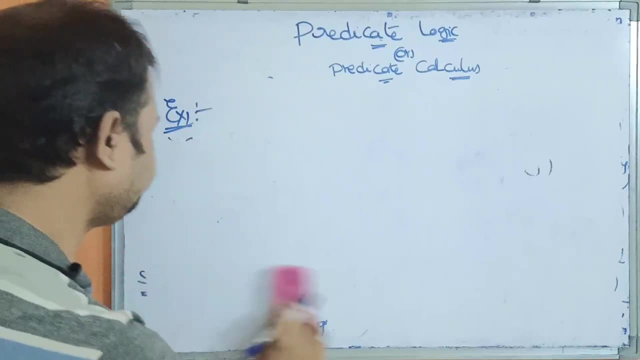 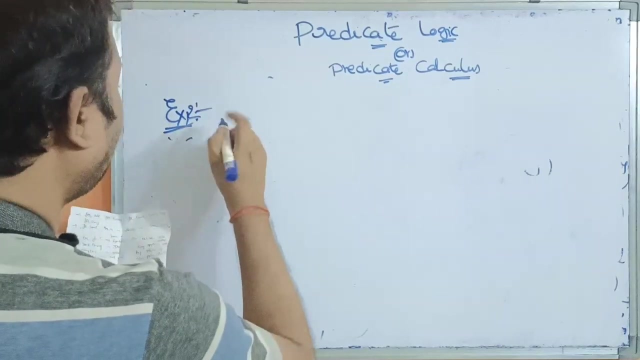 help of the quantifiers in predicate logic. Let us see two more examples. We have two more examples are there? Let us see those two examples Now. let us see example 2.. Let us see example 2.. Let us note down the problem. The first sentence here is: all men are mortal, So mortal means. 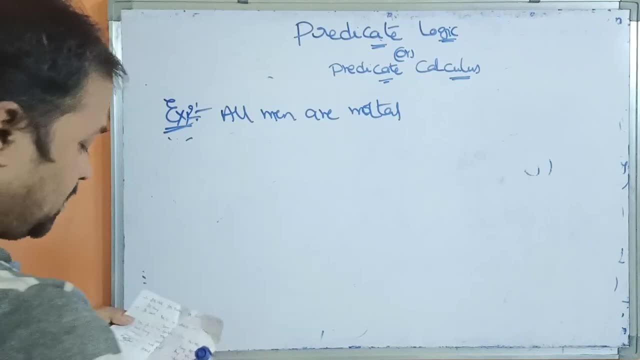 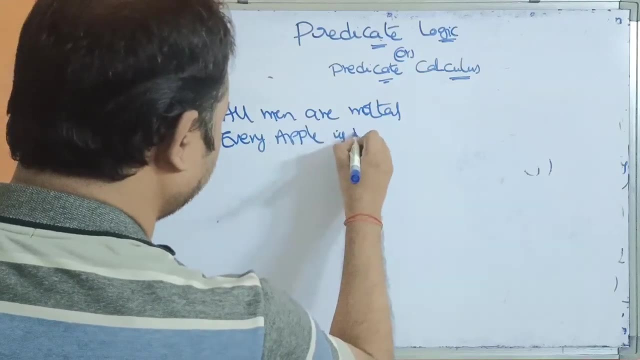 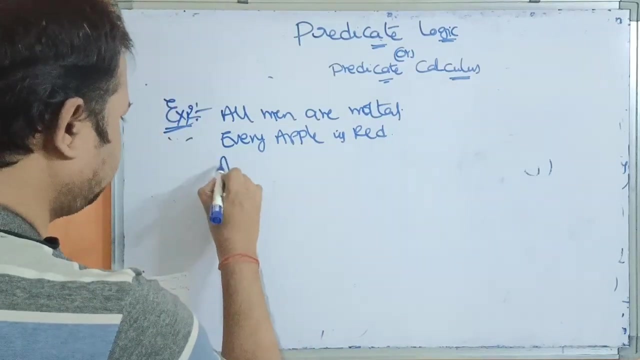 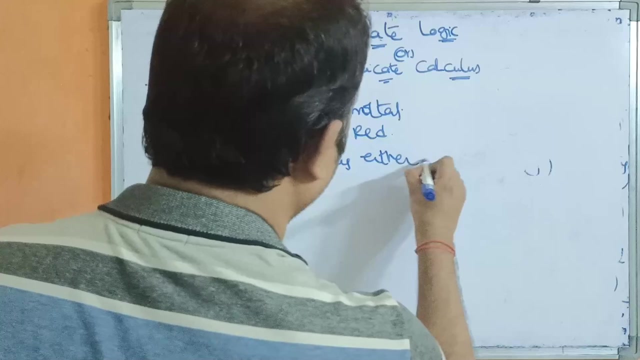 dead. So all the men are dead. Second sentence is: every apple is red. Every apple is red, Every apple is red. Third sentence is: any integer is either positive or negative. Any integer is either positive or negative, Is either positive or negative, Negative. Okay, 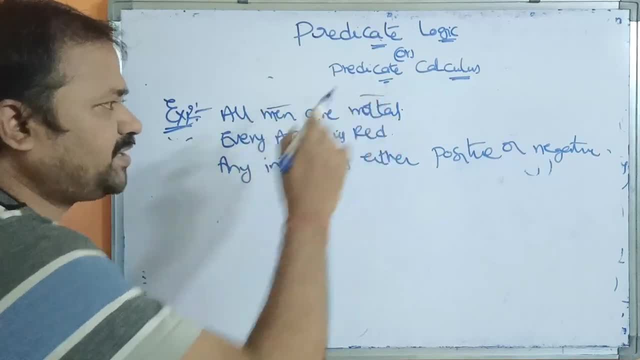 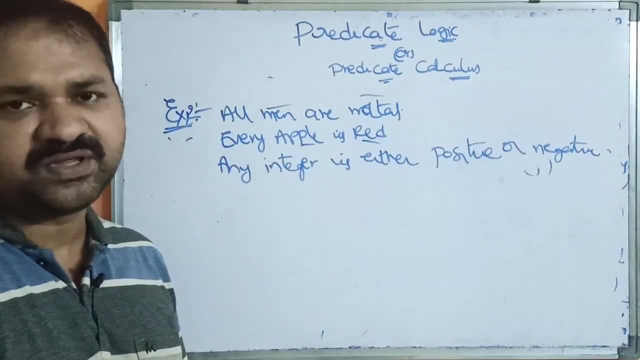 So here, if we consider the first statement, Here we have men mortal, So represent them with the help of the statement function. Here we have yappy, Here we have red, So represent them with the help of the preposition functions. Here we have integer as well as either positive. 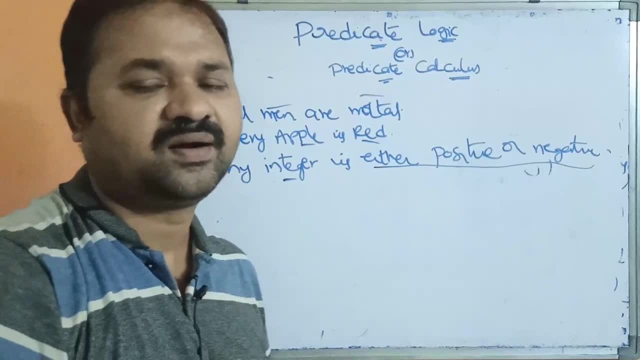 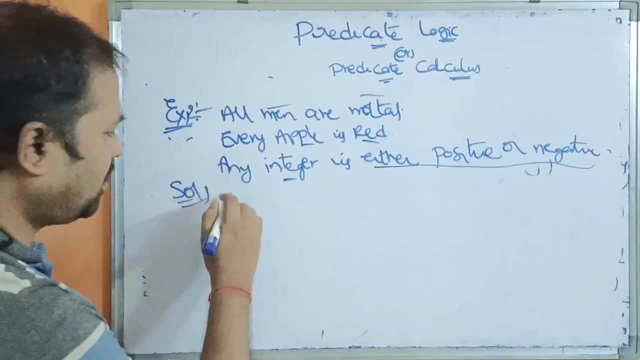 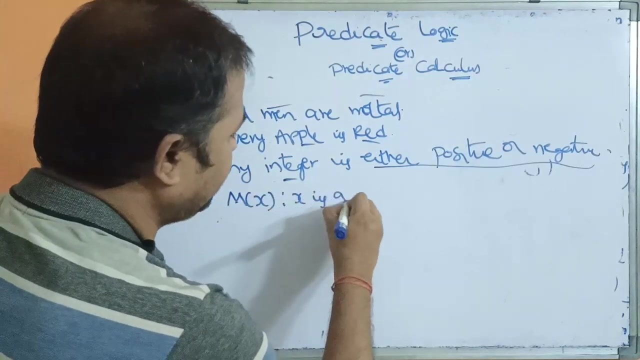 or negative. Let us represent them with the help of the statement function, and then we will write in the sentential form. So what is the first one? All men. So how we can represent men? So men is starting with m, So m of x. x is a man, x is a man. And what is the second? 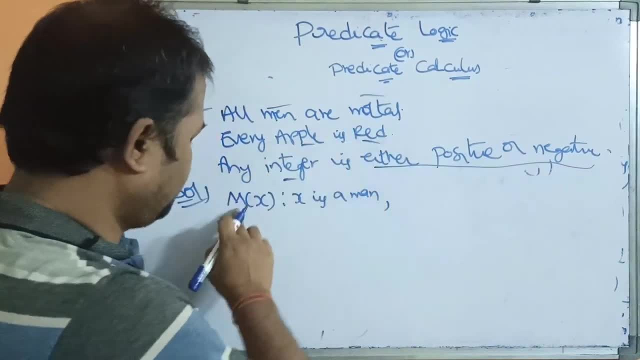 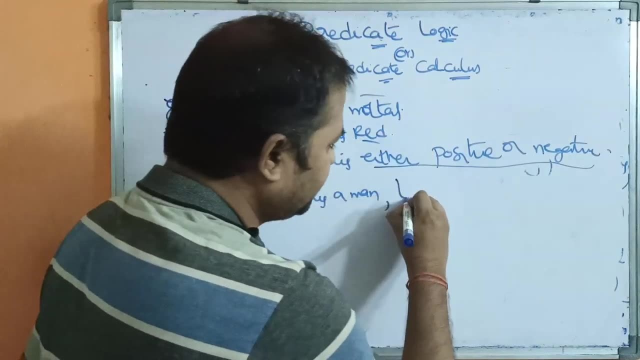 one: Mortal. So mortal is also starting with m. But already we have a statement function which is starting with m. Let us use l here. Mortal is ending with l, So let us use l here. So for space constraints, I am writing here only in the same sentence, But in the examination. 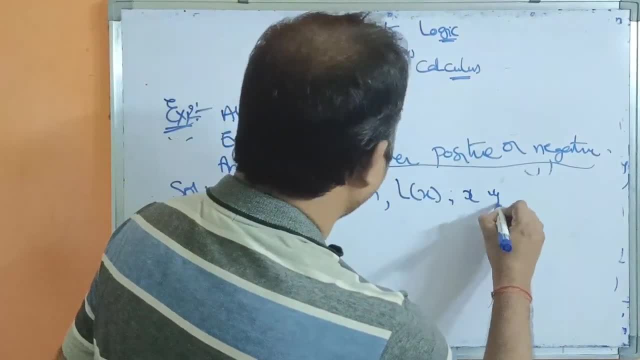 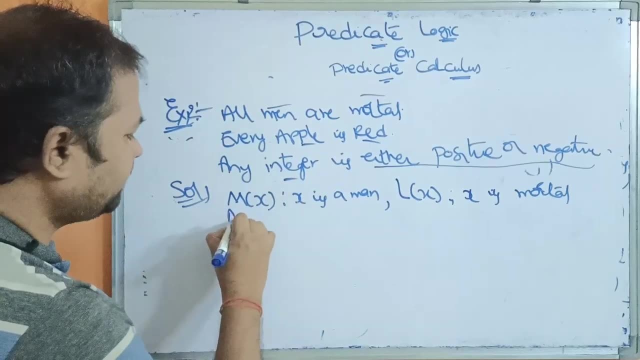 you can write in the next sentence: So m of x, x is a mortal, x is mortal. Let us represent the next one: Yappy. So yappy is starting with a. So a of x, x is yappy, Every yappy. 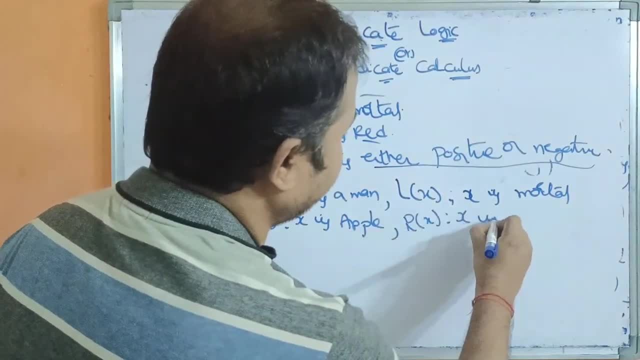 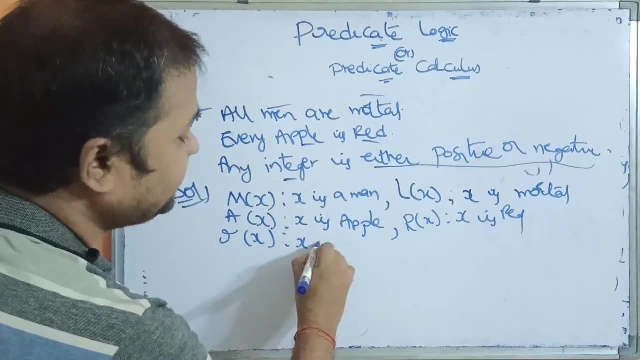 is red, So r of x, x is red. Next one: Any integer Integer is starting with i, So i of x, x is integer, x is integer, So next one: Either positive or negative. So here we have. 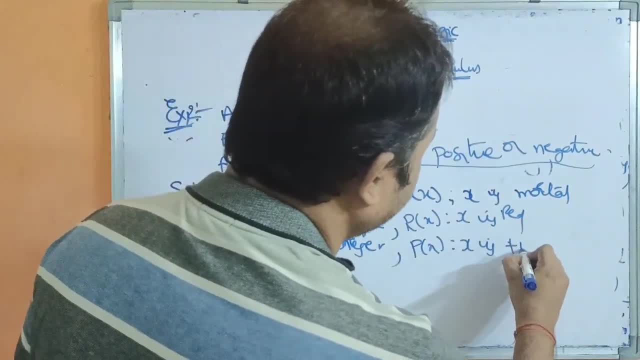 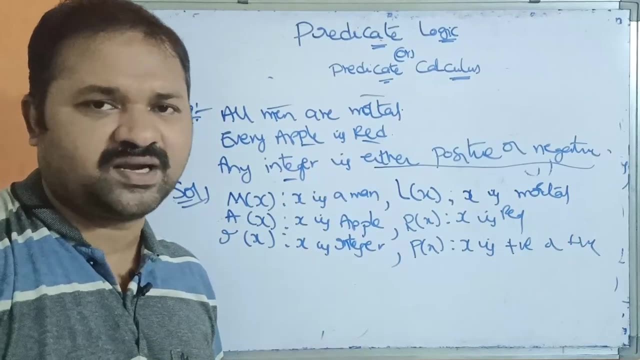 p, So p of x. x is positive or negative. Okay, So let us represent this one: All men are mortal, So every man is mortal. So all means we have to use For all x, For all x. 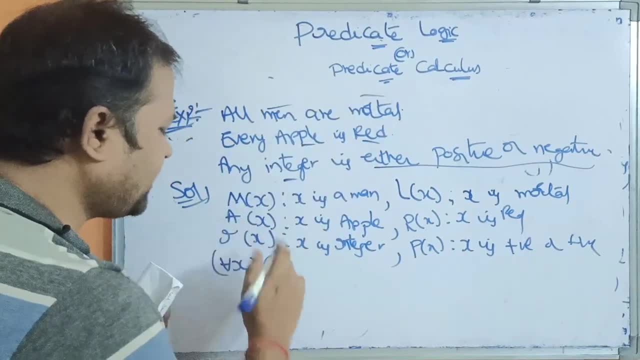 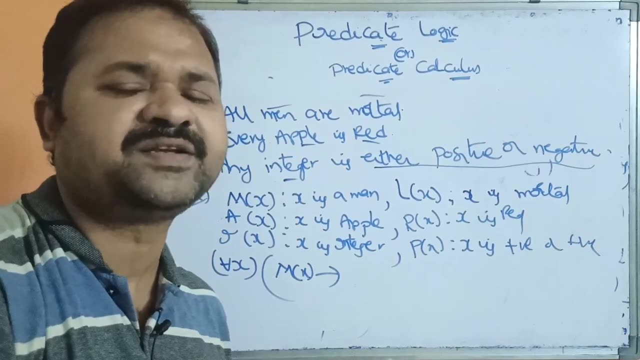 All men, Men, So many, means x is a man, M of x, R, Here all men are mortal, So all men are mortal. Let there are ten men, So all the ten men are mortal. So here we can. 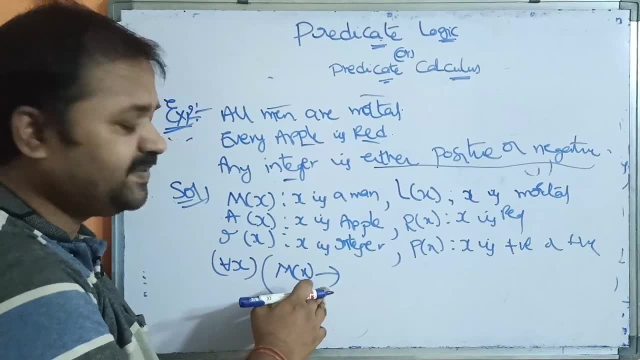 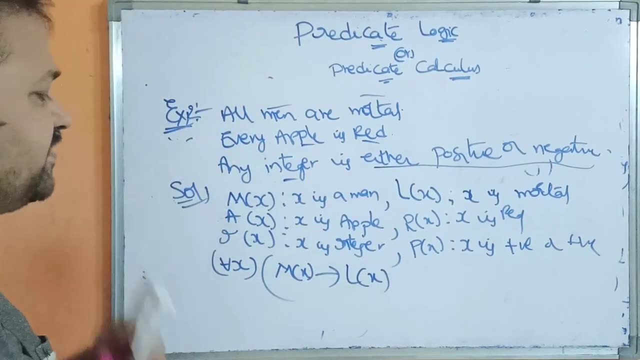 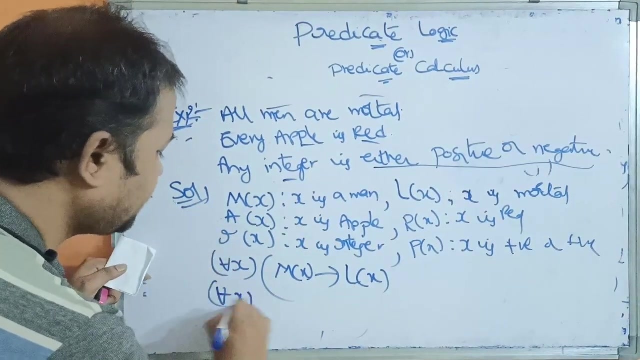 use if, then implication, If, then sentence, That means implication. So mortal means for mortal l, L of x. So we can represent like this Second one: Every apple is red. Every means all Anything. So every means we have to use for all x, Every apple Yappy means. 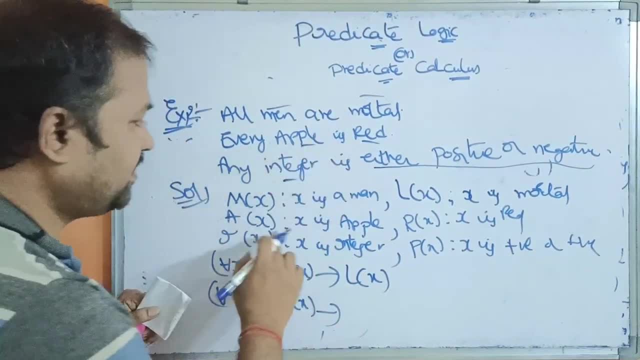 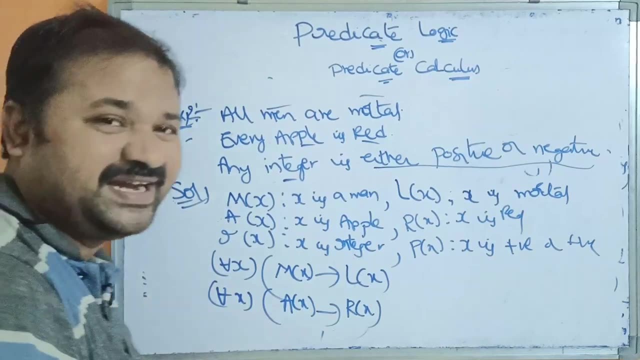 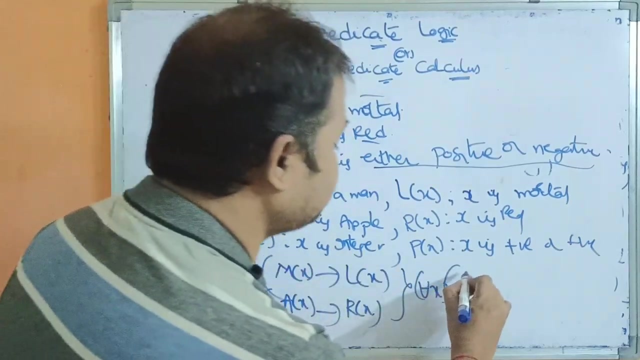 a of x Implies conditional Red. Red means r of x. Let us represent the third one: Every integer, Any integer, So any means every integer, All the integers. Okay, So for all x. Integer means i of x, I of x, conditional x is positive. 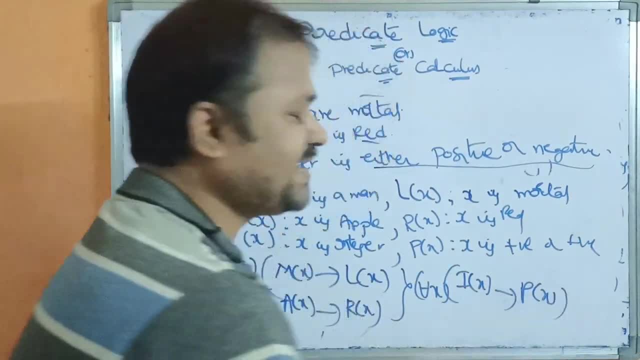 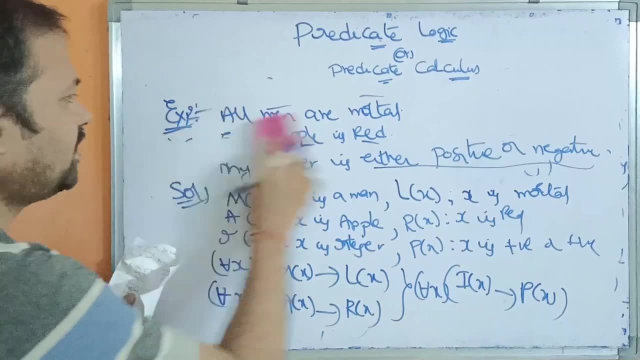 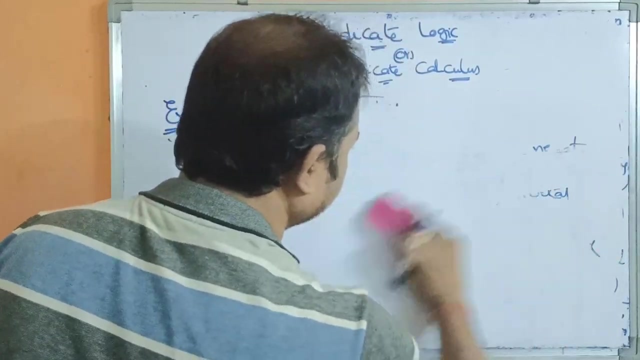 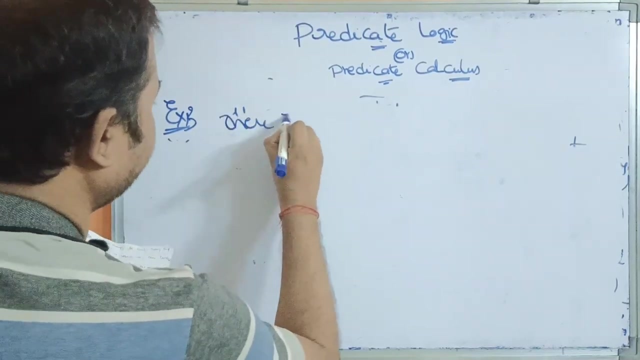 or negative, So p of x. So we can represent like this: Now let us see the last example, Example number three. So last example in this video. So let us see this example, Example two. Example three. Example three: There exists a man. First sentence is there. 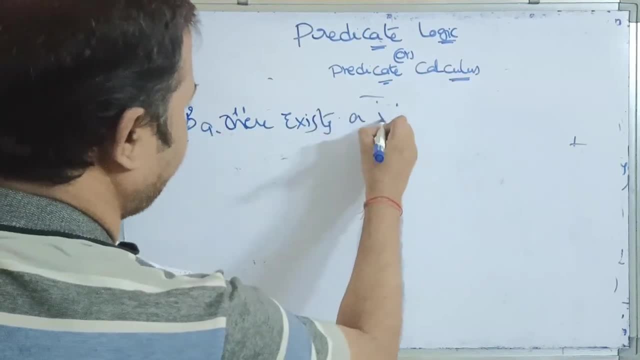 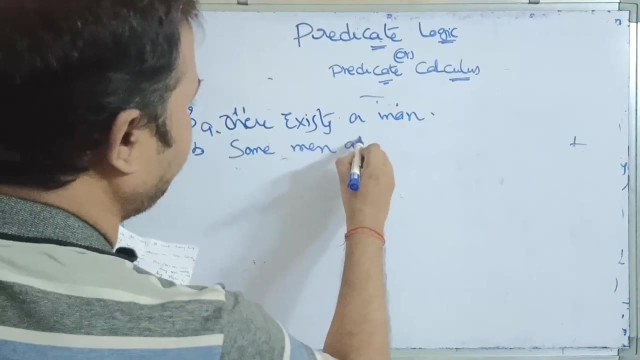 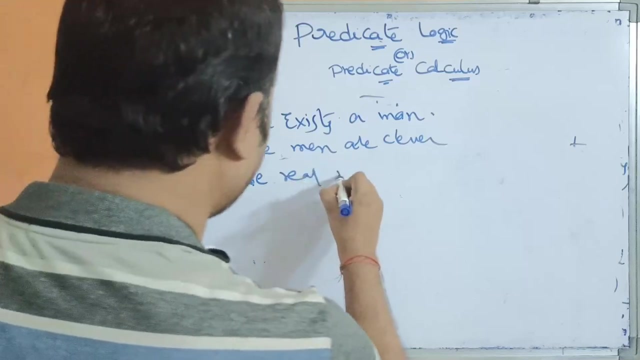 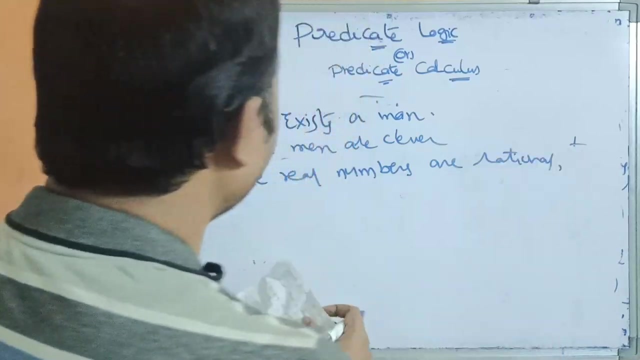 exists. There exists a man. Second sentence is: some men are clever, Some men are clever, Some men are clever. Third sentence is: some real numbers are Some real numbers are rational, Rational. So here in the first sentence we have man. 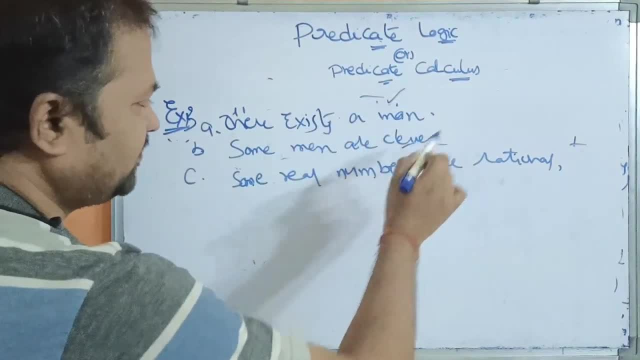 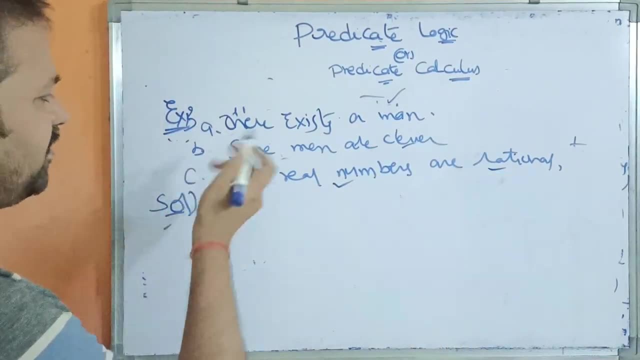 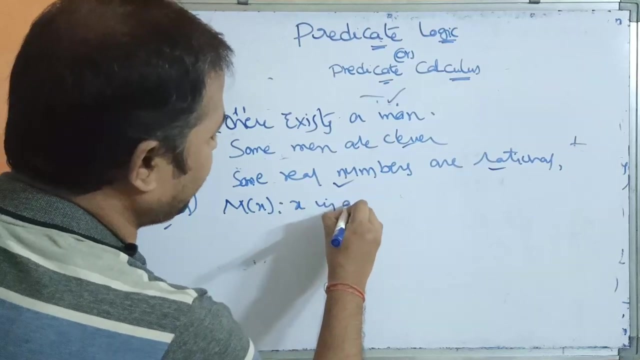 In the second sentence we have man, But he is already represented. So represent clever, Represent real numbers and then represent rational. So first represent them with the help of the functions. Statement. functions So m of x. So m of x means what X is a. 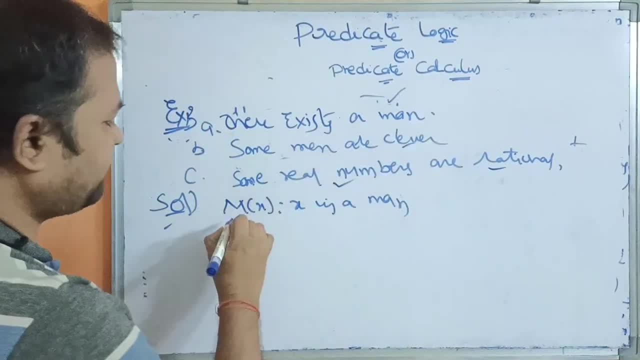 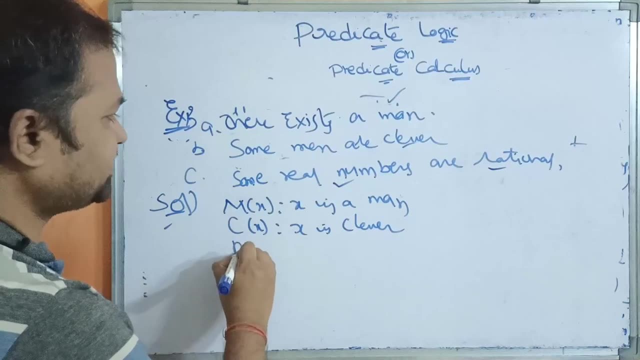 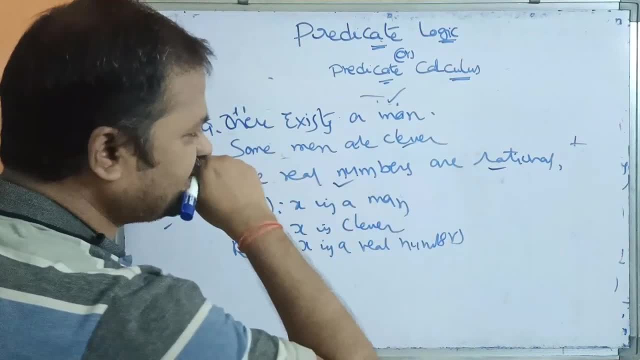 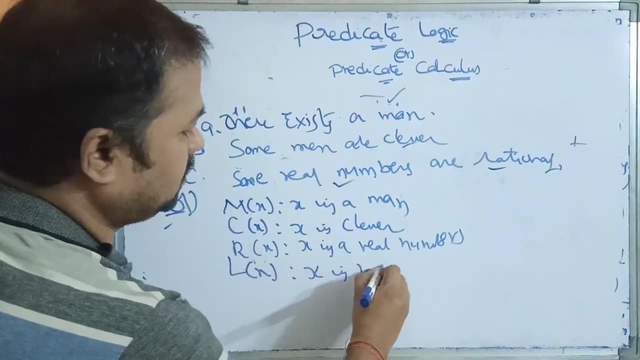 X is a real number, R rational, So rational R is already over. So let us take l, So l of x. X is rational, So let us represent them. There exists a man, So how we can represent. 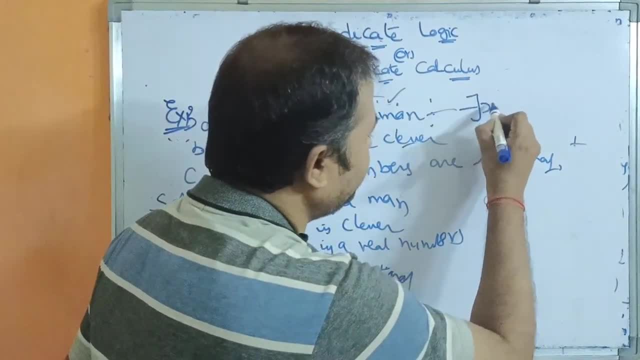 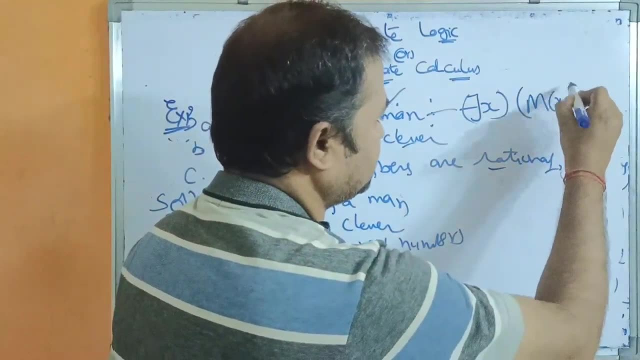 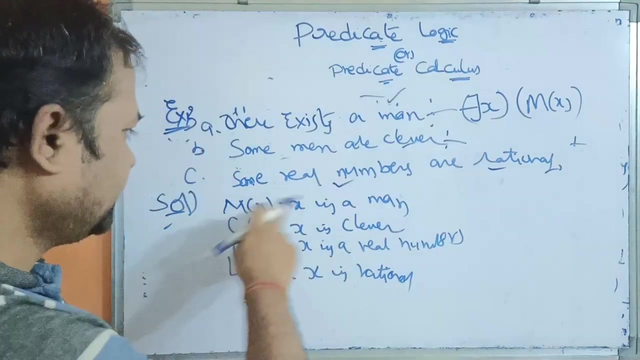 this one. There exists means we have to use, There exists a symbol, There exists a man, There exists x Man. So how to represent man? M of x, M of x. Let us see the second one. Some men are clever, Some men are clever, So how to represent men? So x is a man. 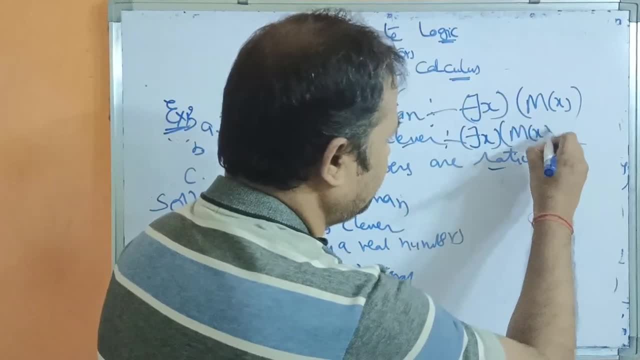 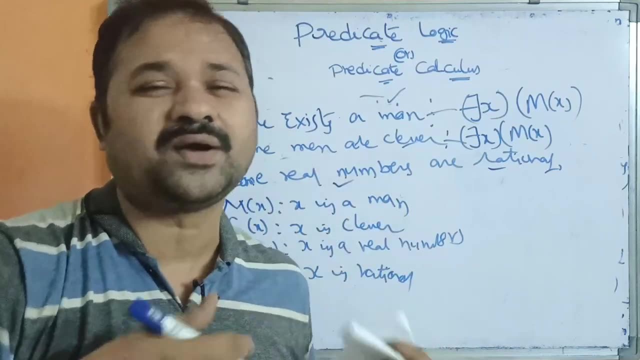 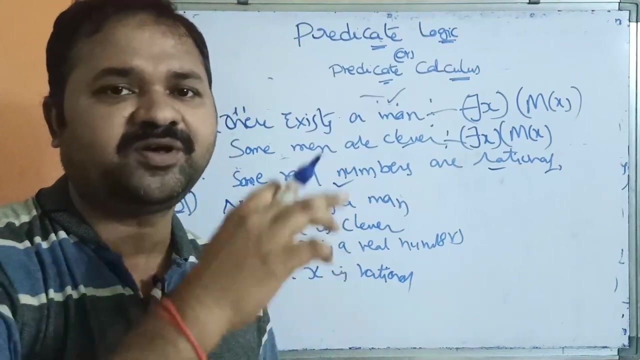 So there exists x, M of x Here. which symbol we have to use? Here we are using there exists, There exists means some, Some, It is not all. If the sentence is all the men are clever, Then we can use implication operator, Conditional operator. Why? Because every man is a clever.